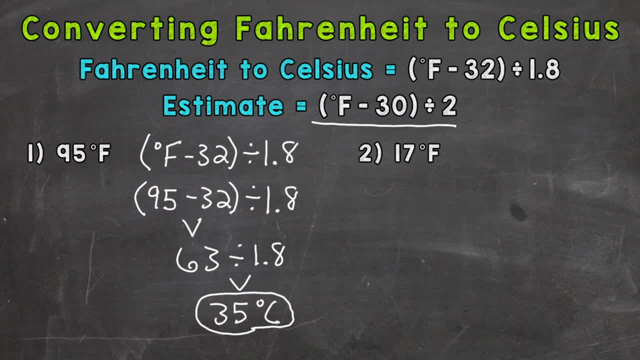 So we rounded the 32 to the nearest 10, 30. And then rounded 1 and 8 tenths to the nearest 10.. To the nearest whole number: 2.. So let's write that estimation formula out So: degrees Fahrenheit minus 30 divided by 2.. 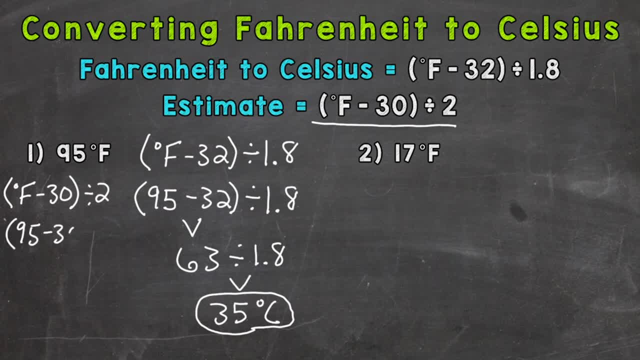 So we'll plug in our 95 here And solve. So 95 minus 30 is 65.. And then 65 divided by 2 gives us 32 and a half, Or 32 and 5 tenths, And that's degrees Celsius. 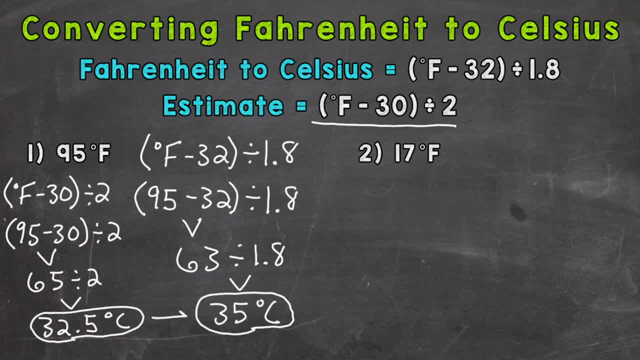 So that is our estimate there, So you can see how it compares to the exact conversion. It did give us a pretty close approximate conversion there. So let's move on to number 2, where we have 17 degrees Fahrenheit. So we will start by rewriting our formula. 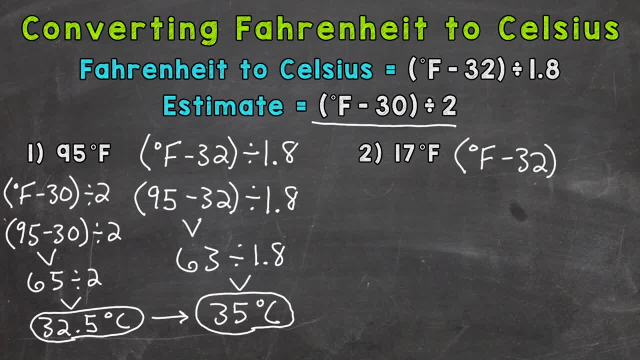 So degrees Fahrenheit minus 32. And then divide by 1 and 8. So we'll plug in 17 minus 32, divided by 1 and 8 tenths. So we'll start by 17 minus 32. Which gives us a negative 15.. 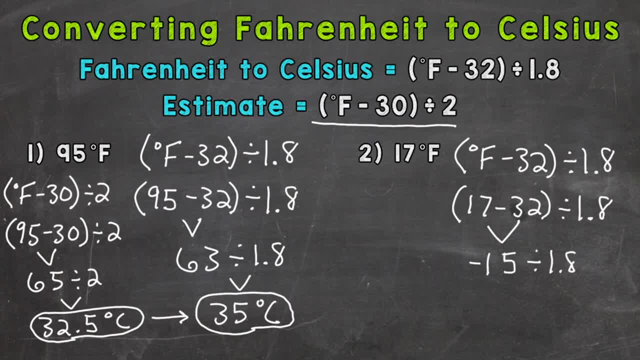 And we will wrap this conversion up by dividing by 1 and 8 tenths. Now 15 or, I'm sorry, negative. 15 divided by 1 and 8 tenths Gives us a negative, Negative 8 and 3 repeating. 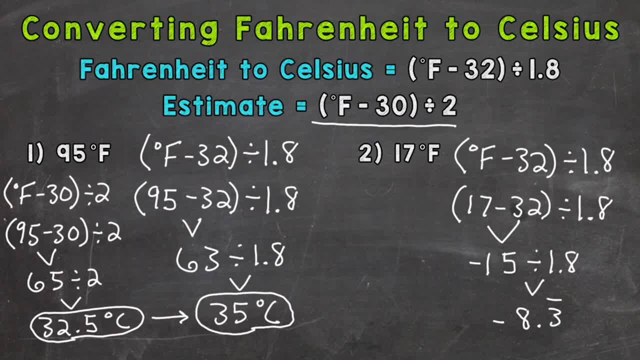 So it gives us a repeating decimal there. So that would be the official way to write it there, With the bar above. the 3 means that decimal is repeating And that is degrees Celsius. So there is our exact conversion. Now we can round that to the nearest whole degree. 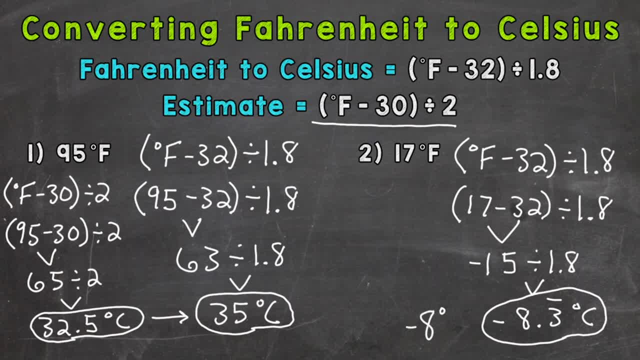 Which would be negative 8 degrees Celsius. So it depends if you want the exact Negative 8.3, repeating or rounded to the nearest whole degree, Which would be negative 8 degrees Celsius. Now, as far as the estimate. Well, let's rewrite our formula here.